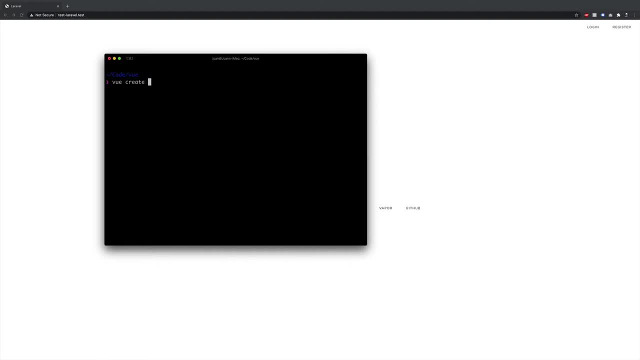 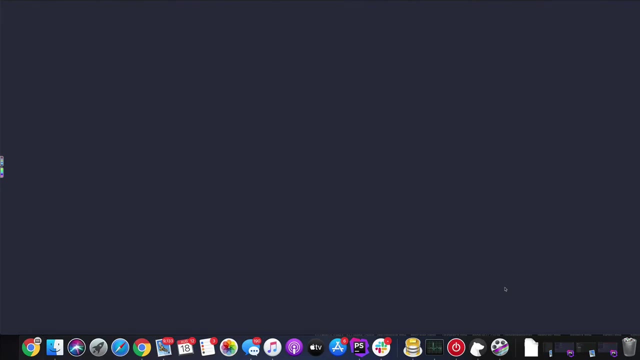 A new view project. So if you create- and I'll just call this YouTube vid- I'm going to install the view 2 and let that finish up. Now that that is done, I'm going to open up PHP storm, I'm going to drag this folder in Create a full screen And I'm going to open up my terminal And I'm just going to run the npm run serve. 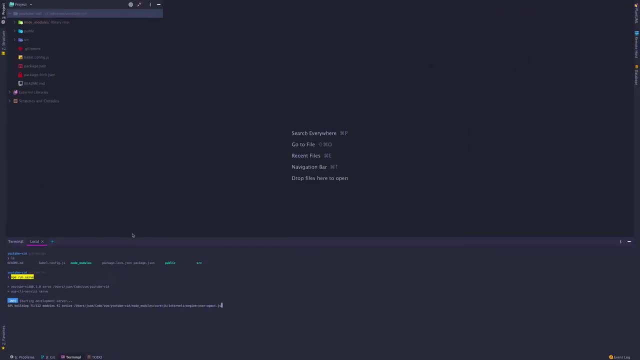 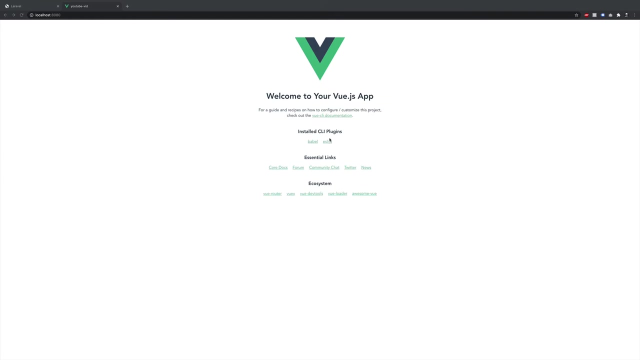 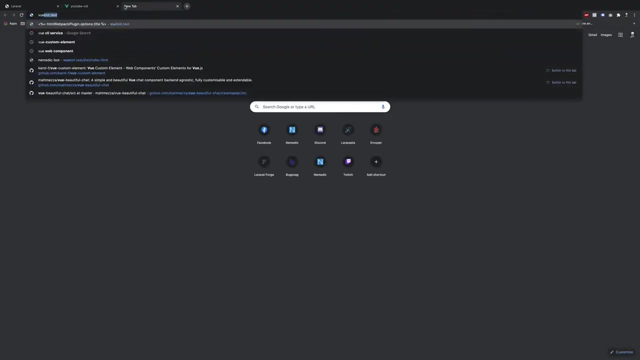 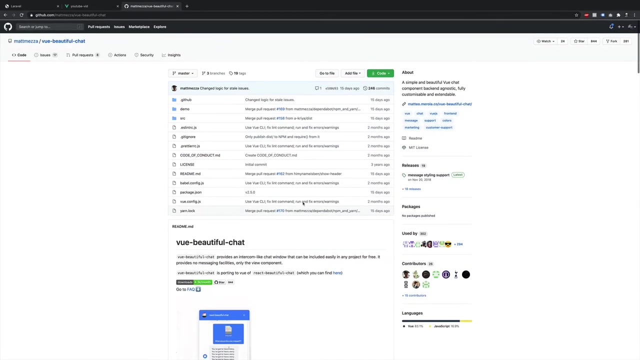 All right, give that a quick look. We don't need the I term anymore, So this is the basic view app here. Okay, so I'm going to use the package, And the package I'm going to use is the view beautiful chat And I'm just going to install this So we can do the npm install. 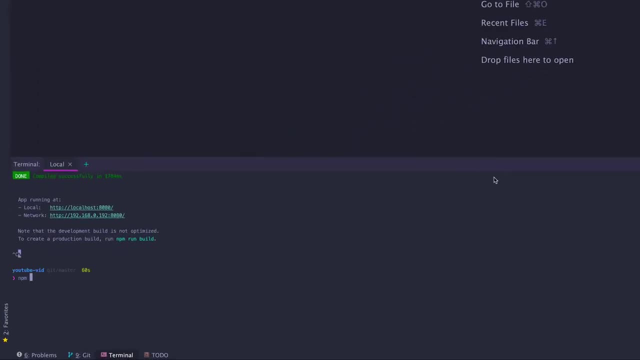 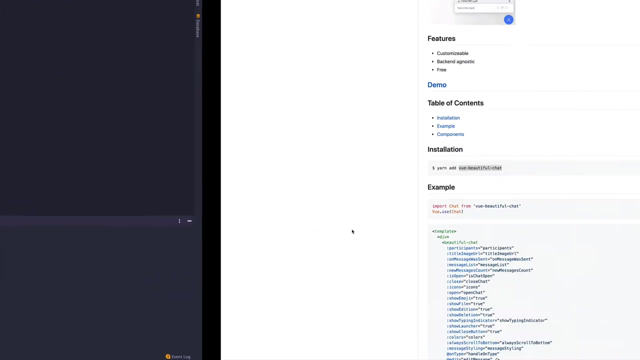 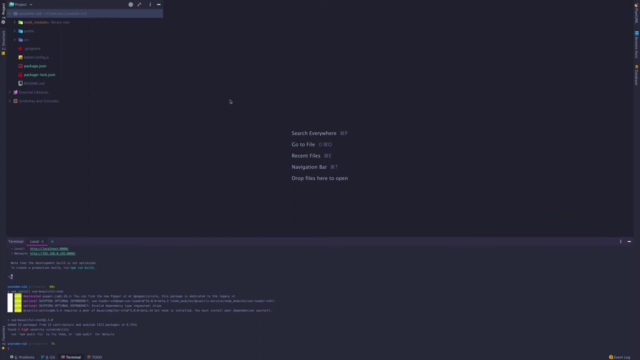 View beautiful chat. So close it off. npm install And let that run. All right, so we're just going to go through the docs here We're going to include, I'm going to report and use in our mainjs file. So under source mainjs we'll go ahead and just pull that in And then in the appvue file we're going to let. 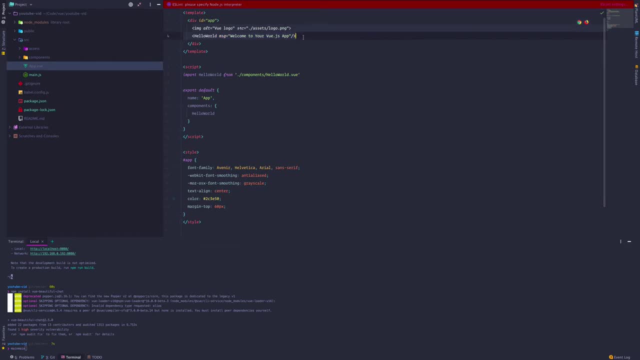 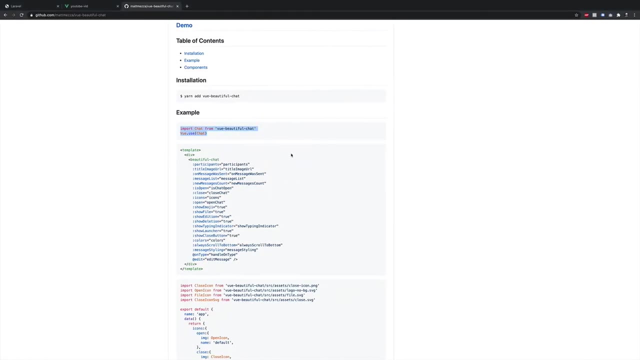 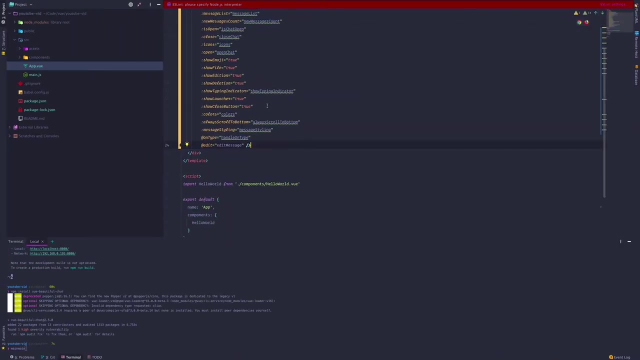 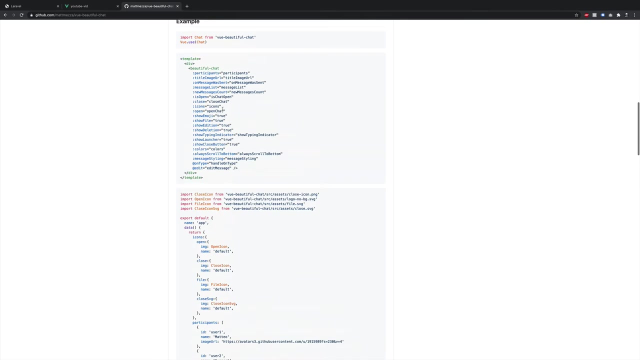 We're going to get rid of all this. We're going to get rid of the content that's in here, Or the styles, And we're going to just pull this over. So I'm going to pull in the beautiful chat component And the script here. So all this up to the export. 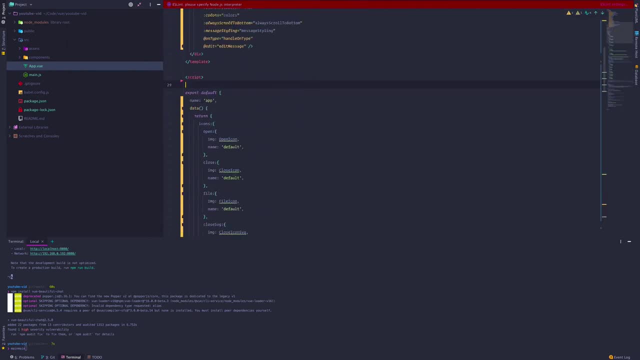 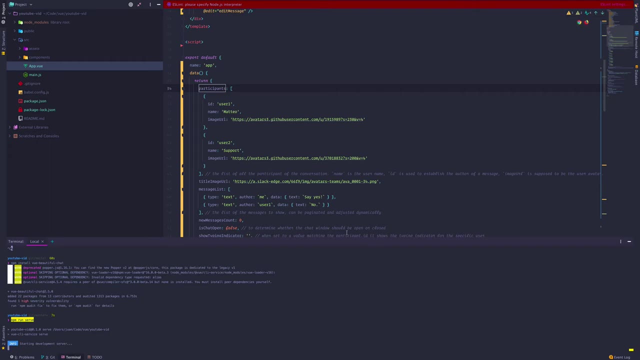 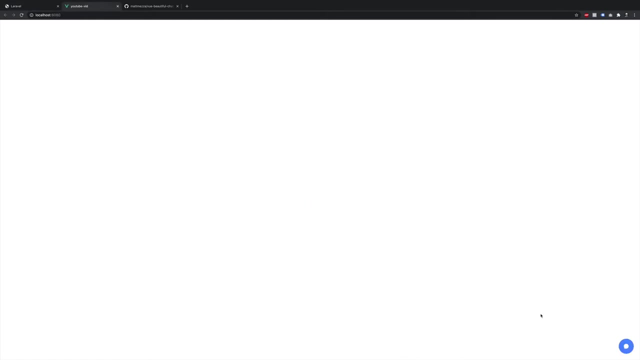 And get rid of this import here And we got to get. got to get rid of these icons So no errors will be thrown, So I'm going to serve that one more time. Probably should let that open. So refresh And we got this component showing correctly. But now I want to use this component on this test Laravel site without having to compile and install. 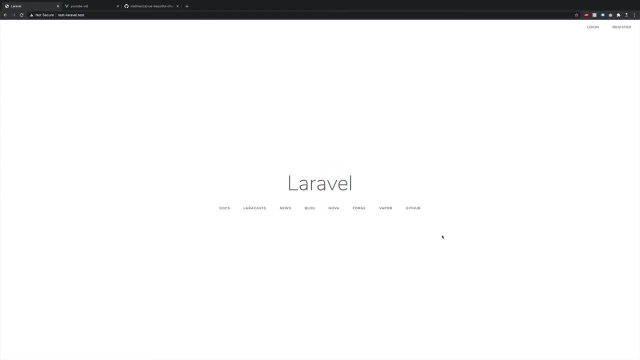 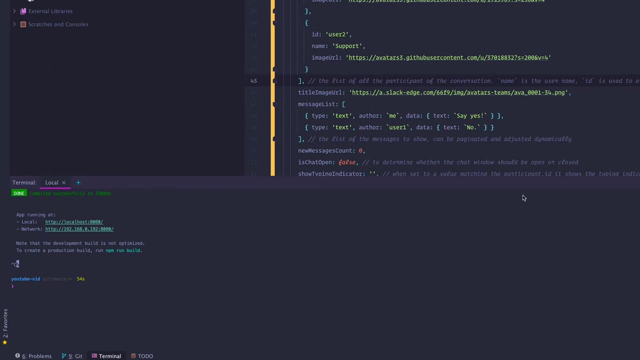 You using the, using the package manager, So this will work on any site, whether it's static HTML or it's Laravel here. So now that I'm back on my project files, I'm going to close that off And since it's working correctly, so I'm going to command view CLI service: build past the target flag of WC. 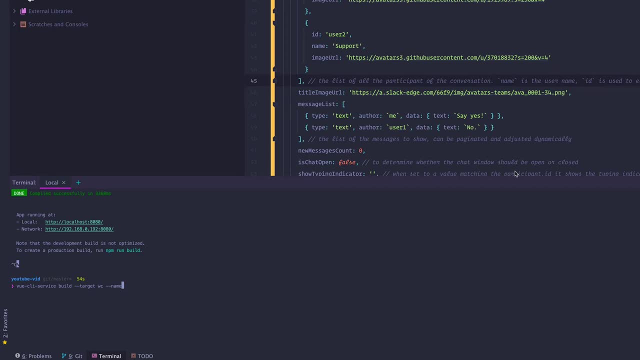 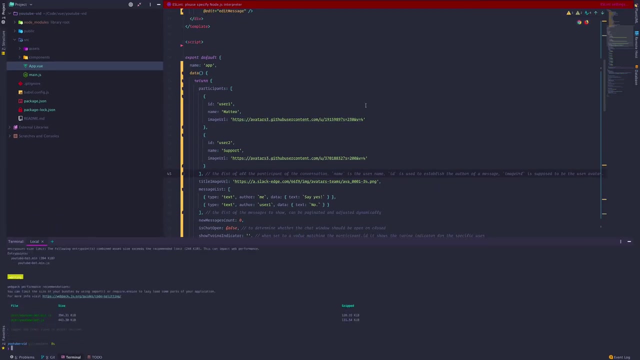 WC is going to be web component Passes the name flag And we'll just call this YouTube bot, And I want to compile down the mainjs file, So let that run. And now we have a distribution file here. So what I'm going to do is I'm going to copy the 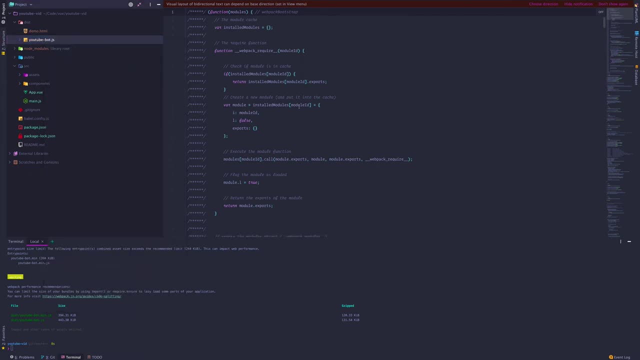 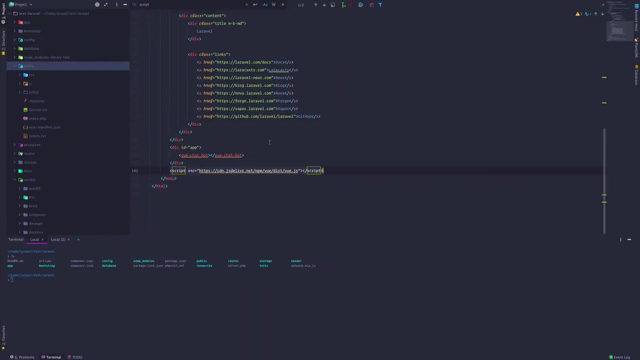 this JavaScript And in this test dot Laravel application here, I'm going to include it here. So, since valet doesn't allow you to load static files without including a driver, all I'm going to do is I'll pull in the CDN package for view here, just above the closing body. So I'm going to go to my public JavaScript. I'm just going to paste in that YouTube botjs file and refresh page. 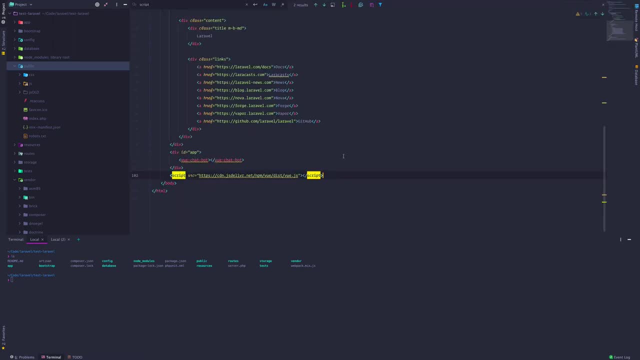 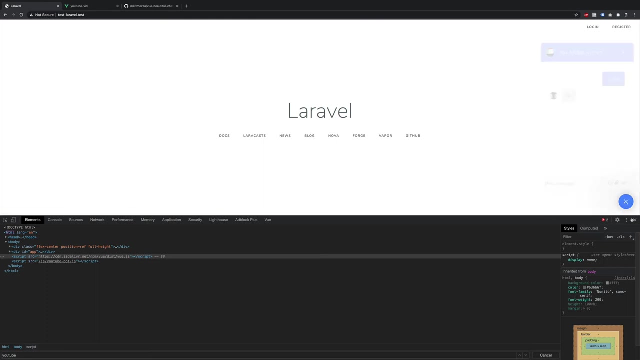 Not showing. so I'm going to inspect the element And I want to make sure I'm on welcome view. I'm going to go ahead and include that script. It's going to be jse2vidjs, I believe that's right. So double check YouTube botjs. Come over here, refresh page. And now this test Laravel application has this: 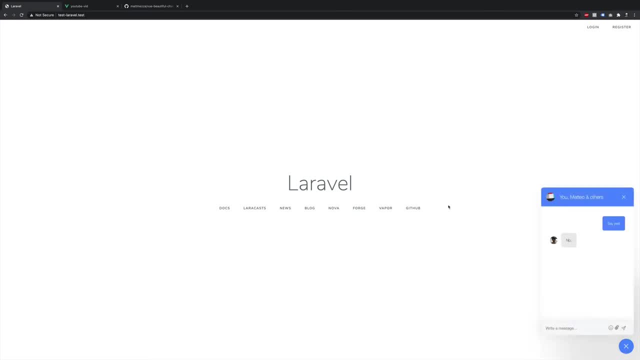 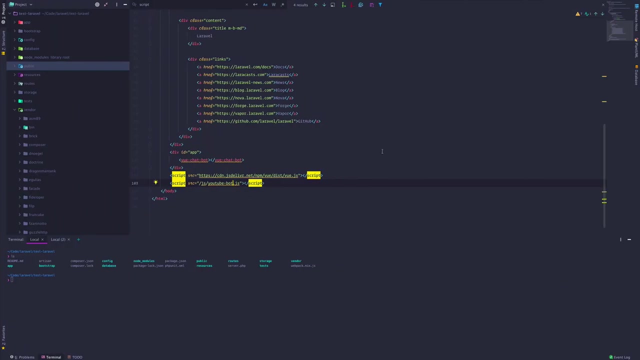 component And it's only including the CDN. So next part is getting it to work with custom components. So I just wanted to walk through that process So I can kind of drill it in my brain And I know I'm going to run to this again. So just basically getting the component ready for a web component, And we didn't pass any data in, We just basically got the shell taken care of. So now we come back to the main project here, the view project.